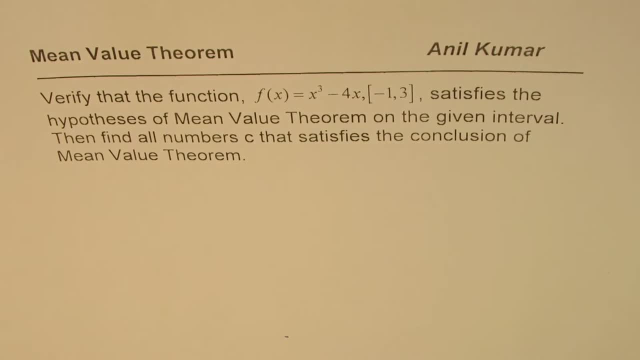 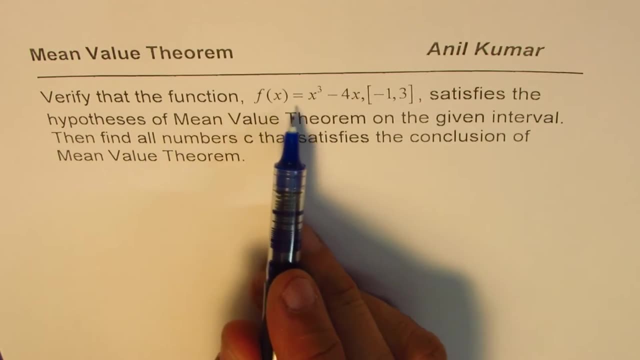 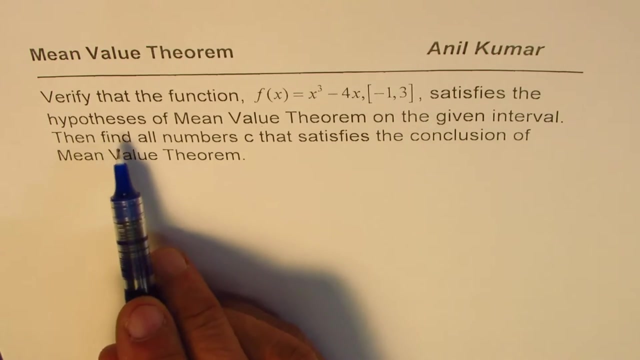 I'm Anil Kumar and here is an example to illustrate mean value theorem. The question is: verify that the function f of x equals to x cubed minus 4x in the closed interval minus 1 to 3 satisfies the hypothesis of mean value theorem on the given interval. 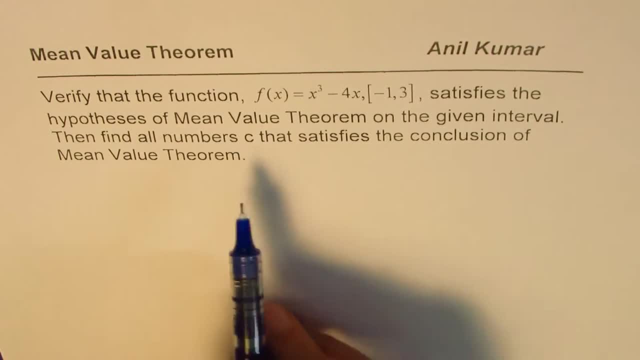 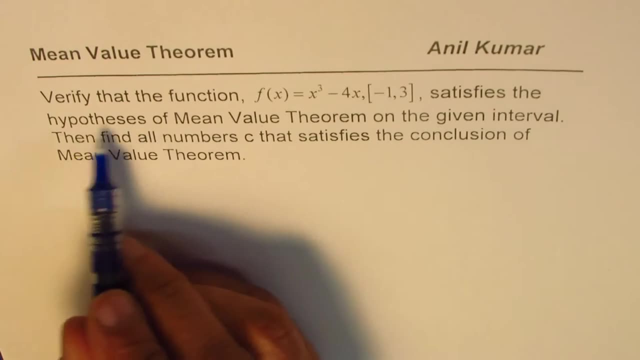 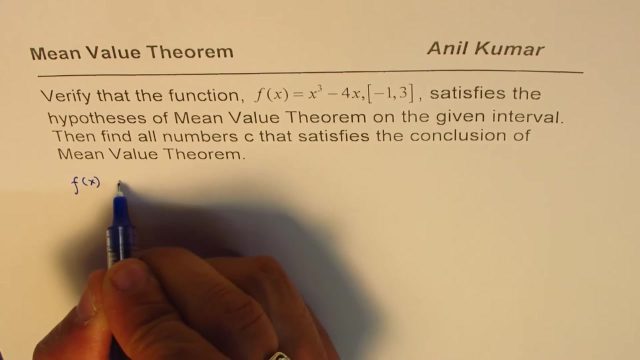 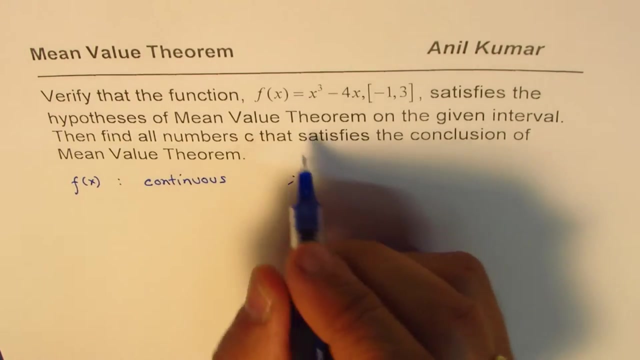 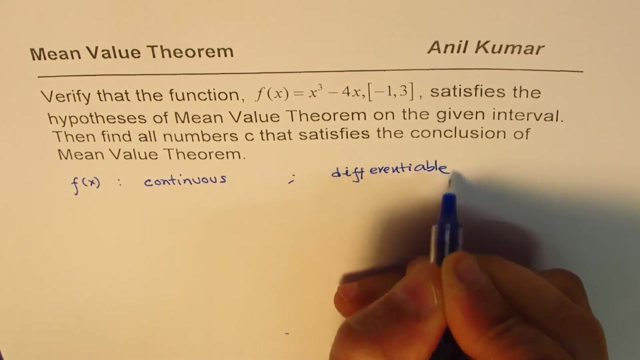 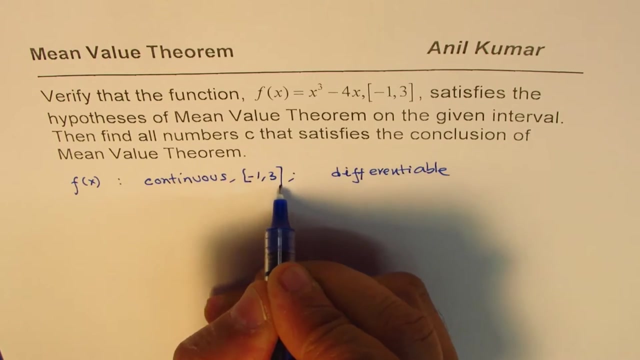 Then find all numbers c. that satisfies the conclusion of the mean value theorem. Now, to satisfy the hypothesis, we have two hypotheses. One is regarding that the function f of x should be continuous and the other one is that it should be differentiable. Now it has to be continuous in the closed interval, which is given to us as minus 1 to 3, and it has to be differentiable in the open interval, minus 1 to 3.. So these are the two conditions. 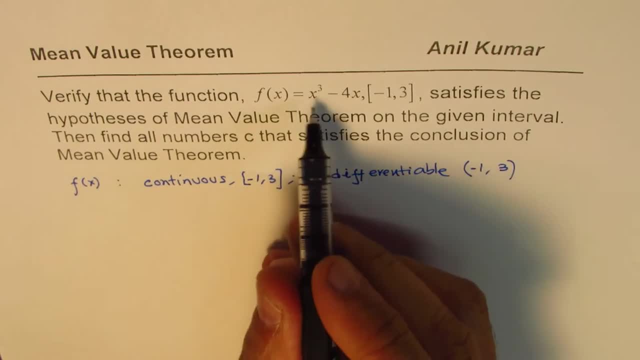 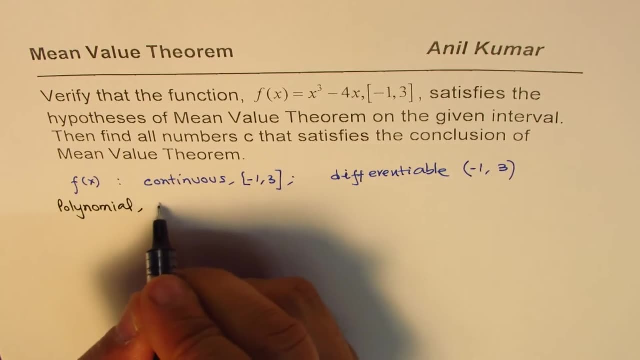 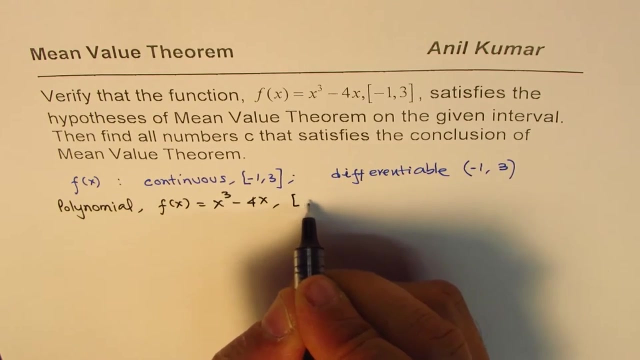 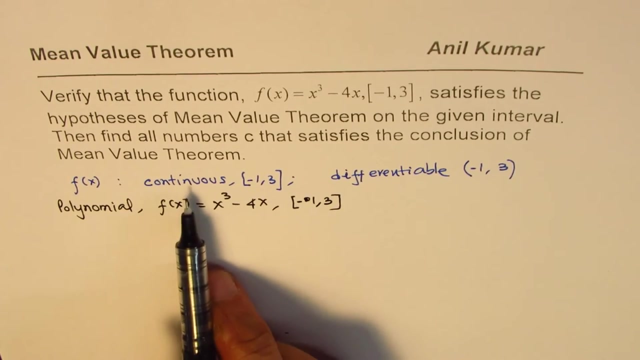 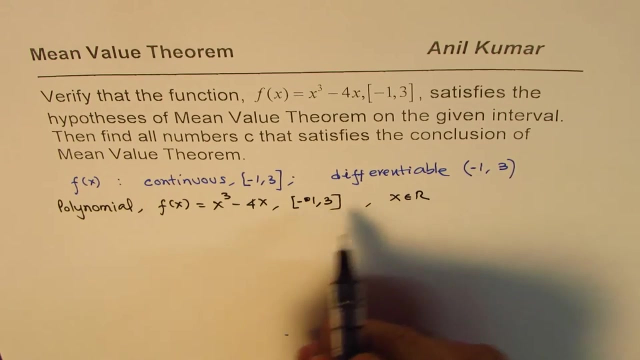 Now, since the function given to us is a cubic function, it's a polynomial, right? So we have a polynomial which is f of x equals to x cubed minus 4x, And we're talking about the closed interval from minus 1 to 3.. Okay Now, since polynomial is a continuous function and differentiable in its domain- x belongs to real numbers- it is also continuous and differentiable within the given domain, right? So that's the kind of proof we can say that satisfies hypothesis of mean value theorem, right? So that's the first one. 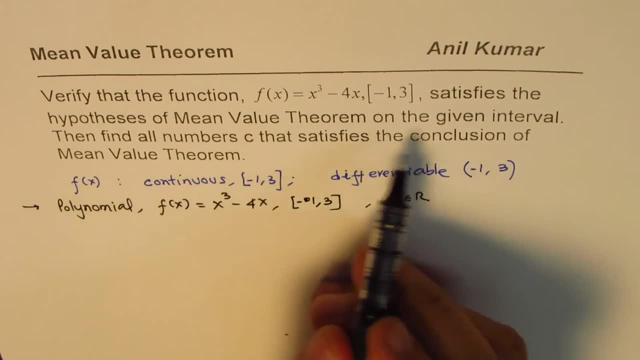 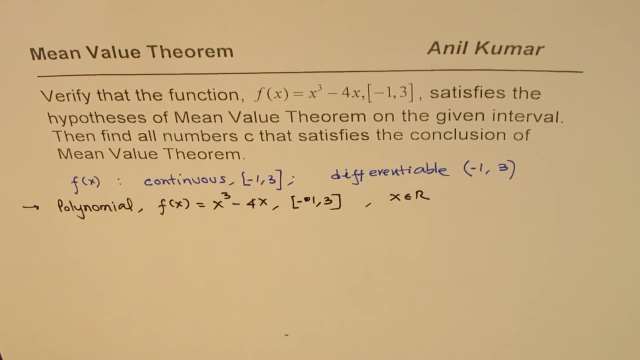 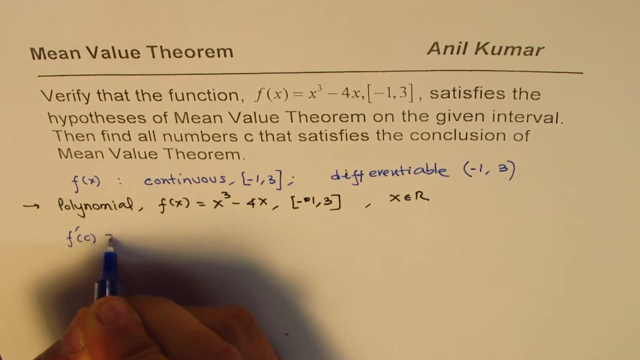 Now second part of the question is then: find all numbers c. that satisfies the condition of mean value theorem. Now, what is the condition of mean value theorem? The condition is that f dash c should be equal to f of b minus f of a divided by b minus a. So that is the condition. 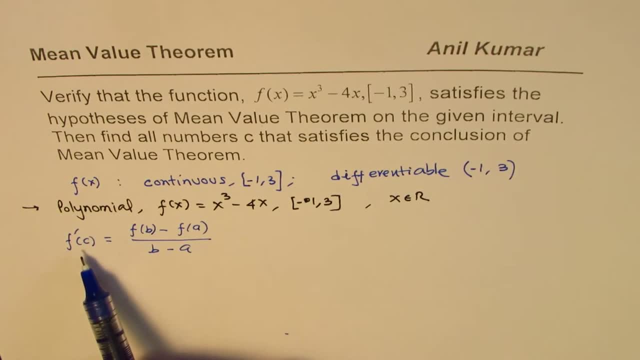 Sometimes we say that the instantaneous rate of change in the function f of x is equal to f of b minus f of a divided by b minus a. So that is the condition. But the moment that the points are methyl, f are hadlous, f are hadlousso, the total range at some point within the open interval is same as the average rate of change between the two points in the interval. right? So that is what it is. 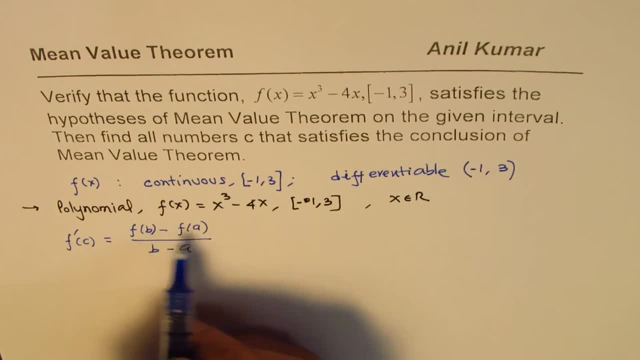 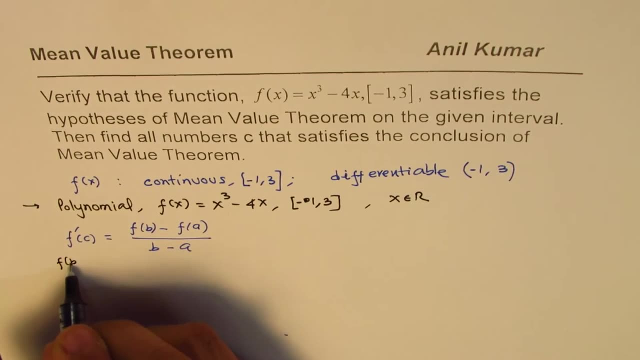 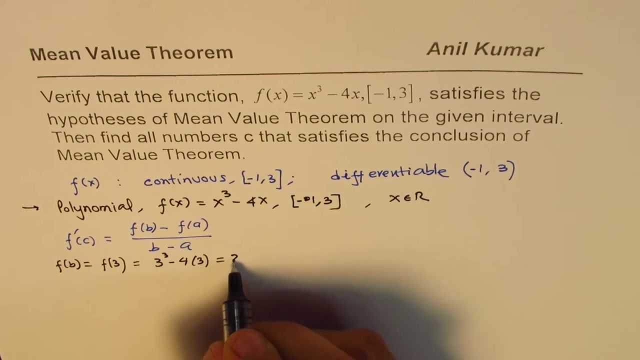 So in our case we can find what f and f are, substitute the values and then calculate right. So f of b is equal to 3, which is f of 3.. So if I substitute 3 here, we get 3 cube minus 4 times 3, that is 27 minus 12, minus 12, so that is 5, 15, right. 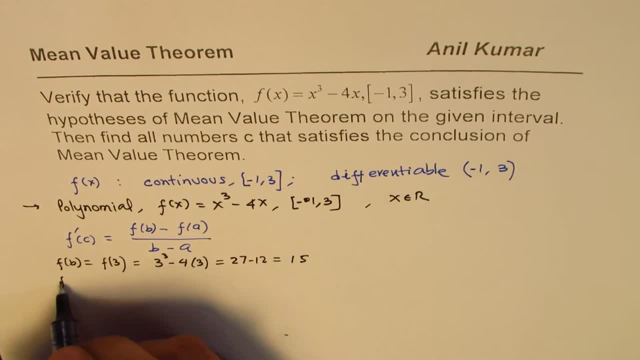 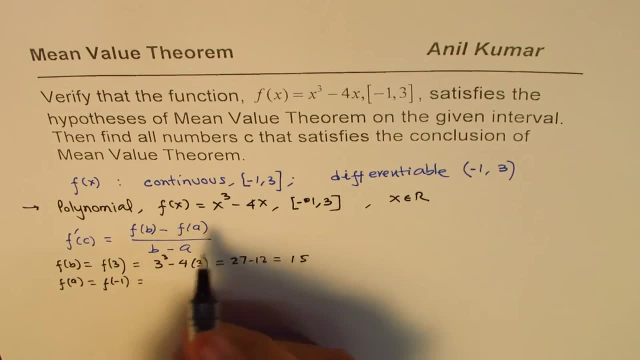 So 27 minus 12 is 15.. And let's find what is f of a. a in this case is minus 1, so f of minus 1, which is minus 1 cube minus 4 times minus 1.. 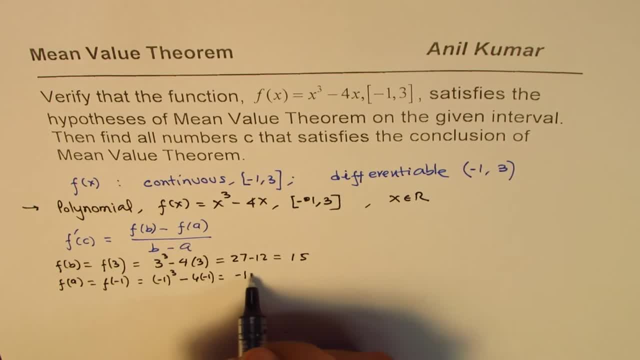 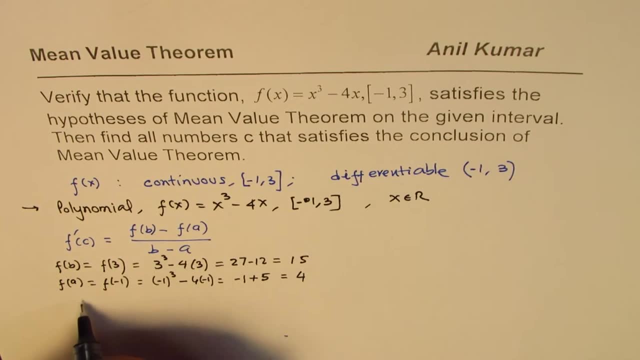 So that is minus 1 and that is plus 5, so that is 4 for us, right. So from here we can say what should be f dash c equal to. So f of b is 15, so we will do 15 minus 4 divided by 3 minus minus 1, 3 minus minus 1, right. 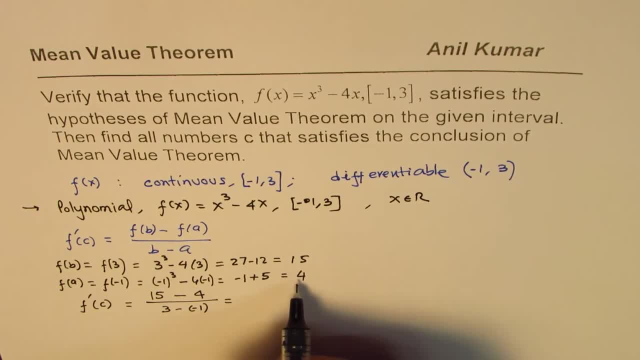 So that is 15.. 15 minus 4 is- I think I did a mistake here- 4 times minus 1 was not 5, but 4, right, So let me correct this. Good time to check it. 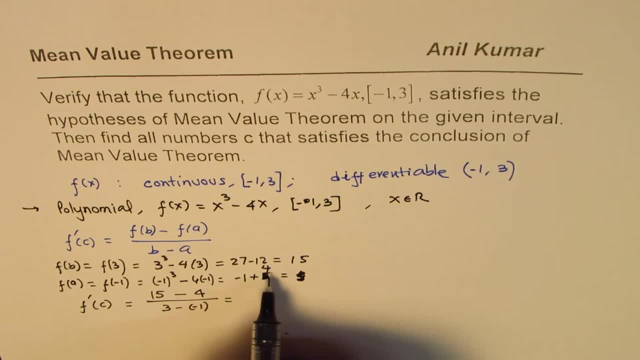 So we have minus 1 plus 4,, which is 3,, right So, which is 3.. So this value is not 4,, but 3, okay, Minus 1 plus 4 is 3.. 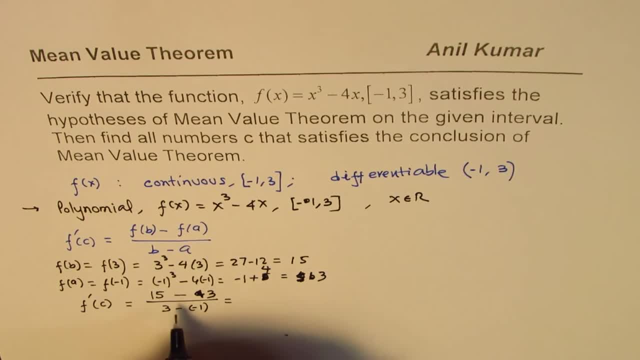 So we have 15 minus 3 divided by 3 minus minus 1.. 15 minus 3 is 12, so we get 12 divided by 4, and that gives us 3.. So the value of f dash c should be 3.. 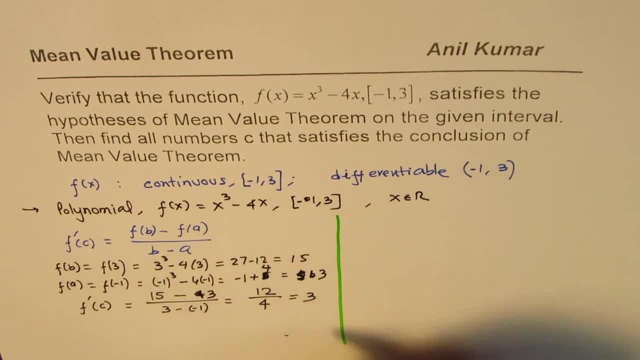 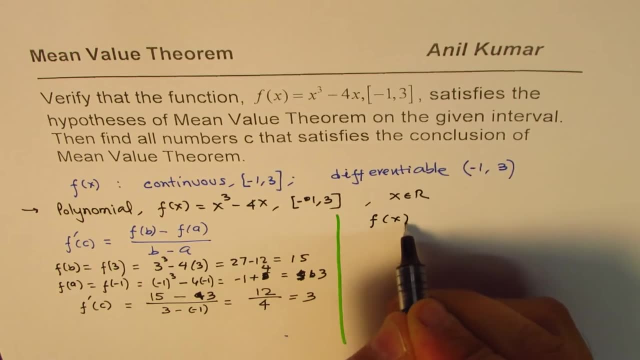 Now to find what c is. we can actually find the derivative. equate it to 3, right. So what we are given here is the function f of x equals to x cube minus 4x. So f dash x. 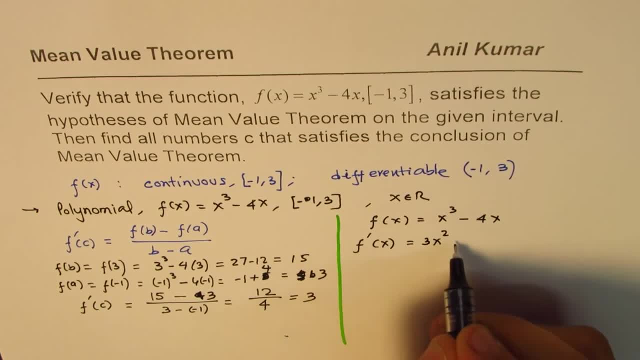 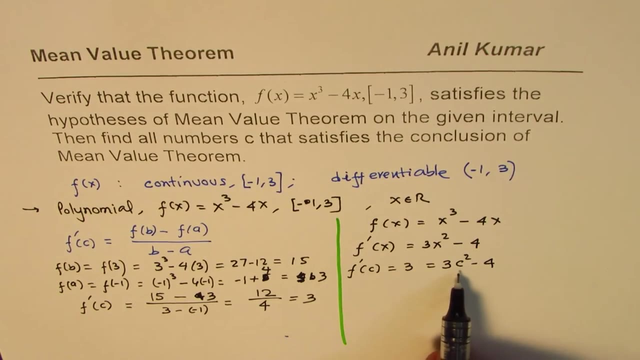 f dash x is equal to 3x square minus 4.. Now, since we know that f dash c is equal to 3, we can write c here, So we have 3c square minus 4, and find what c is right. 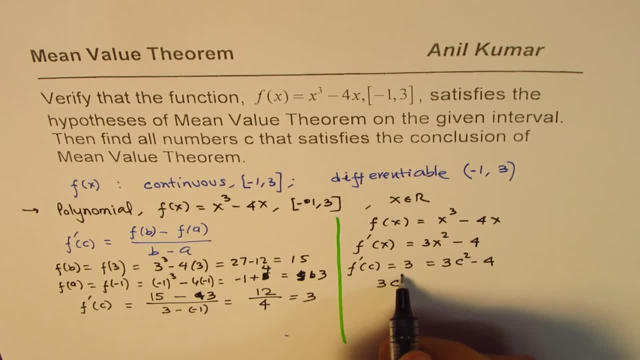 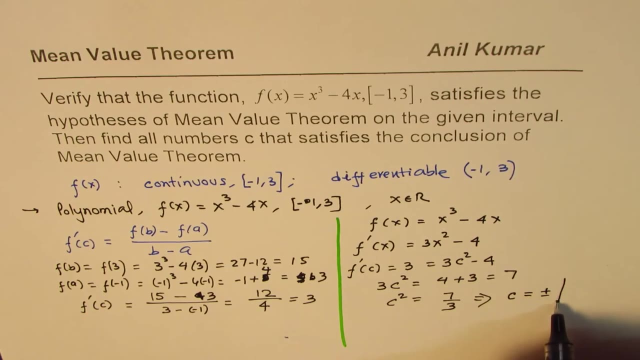 So we'll just rearrange it So we can write: 3c square is equal to 4 plus 3, which is 7.. c square is 7 over 3.. Or this implies that c is equal to plus minus square root of 7 over 3.. 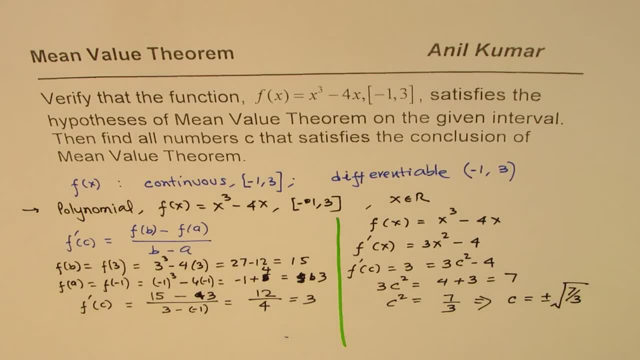 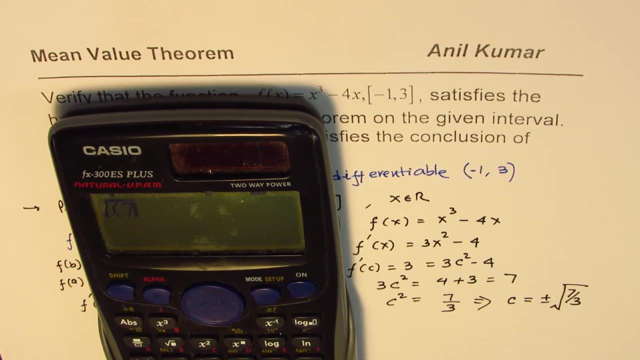 So that becomes the answer. Now we need to check whether these values are within this interval or not. right, So we can just take the calculator and calculate this value. So we have square root of. let me write within brackets: 7 divided by 3, bracket close. 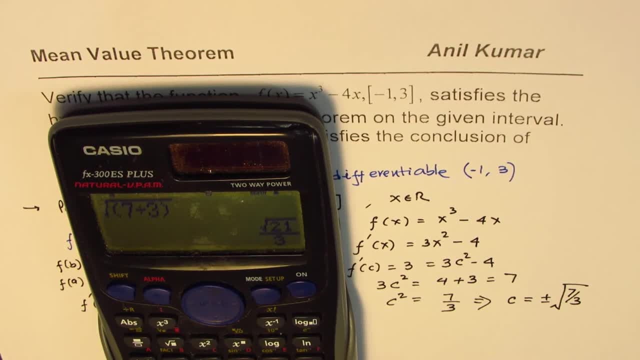 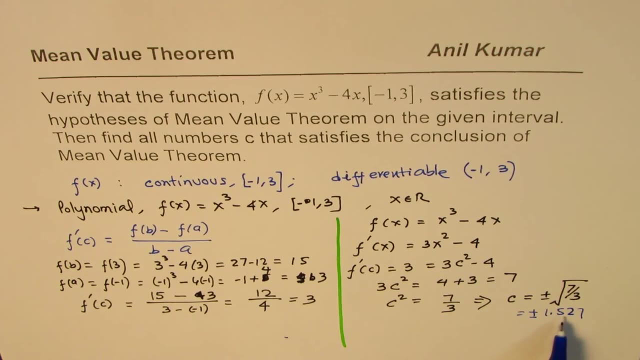 equal to, So that in decimals is equal to plus minus 1 point approximately. Let's say, let me write 5 to 7.. How does it matter? So plus minus 1 point 5 to 7, right. 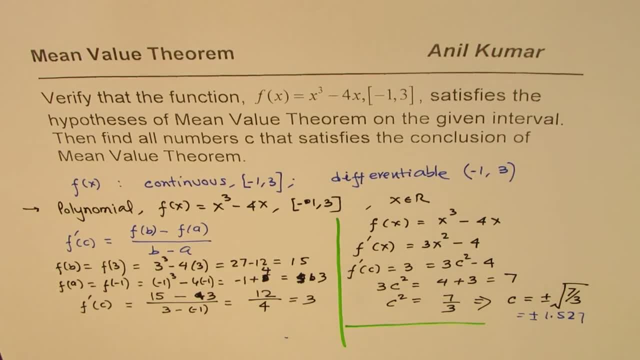 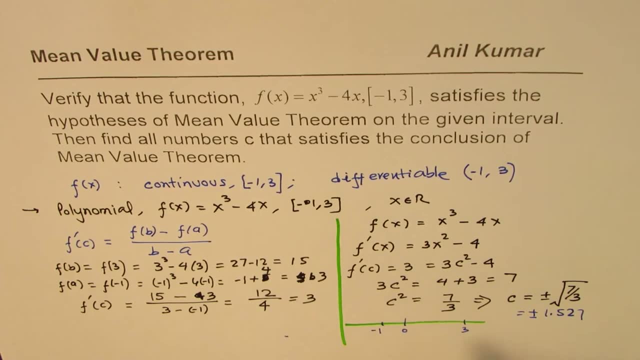 So on a number line, you can see that on a number line if we have 0 here and let's say this is 3, and this is your minus 1. Then plus 1, point 5 is kind of in between somewhere. let's say here: right? 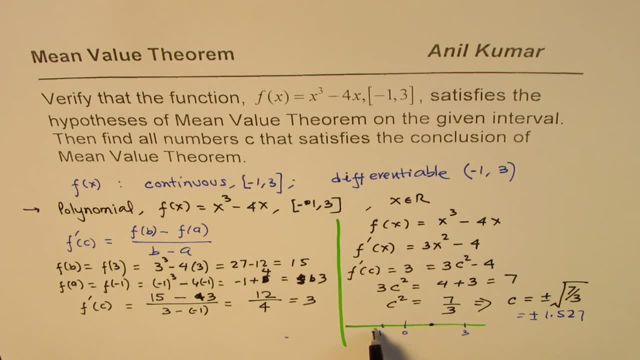 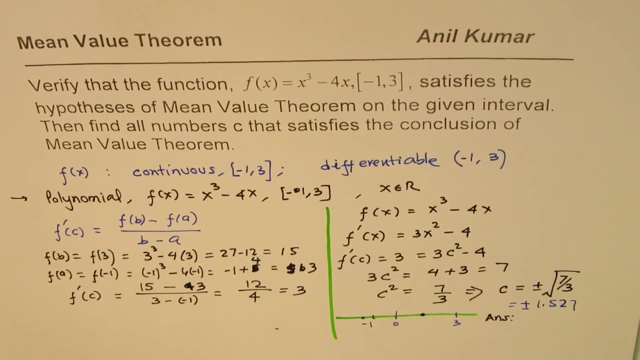 So, and the minus 1 point 5 will be outside our domain, right? So the value of c which really satisfies the answer is: is the plus value, right? So what we get here is that answer is: c is equal to 1 point 5 to 7.. 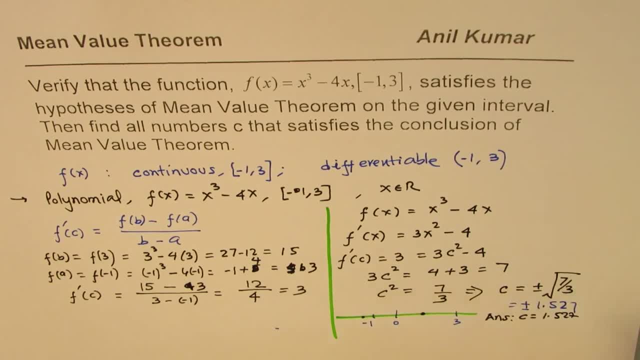 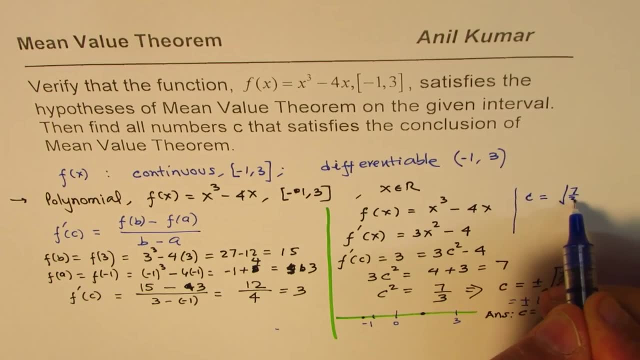 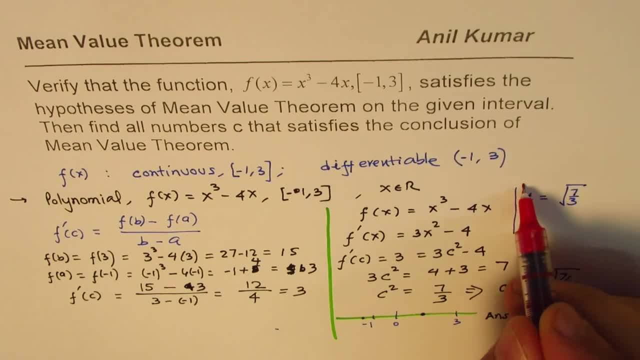 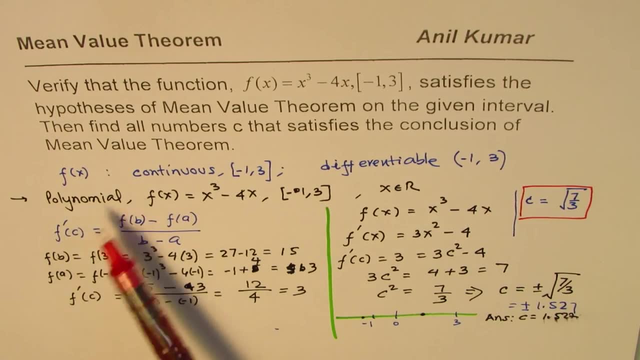 So that becomes the solution for the given equation, right? So that is the answer. So I hope you understand how we figure it out. So one: we prove that the conditions are met, the function is continuous and differentiable.